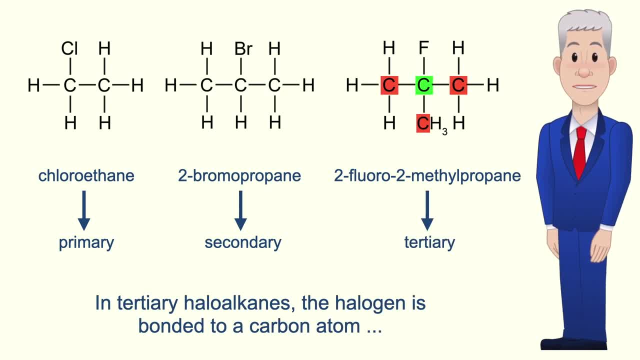 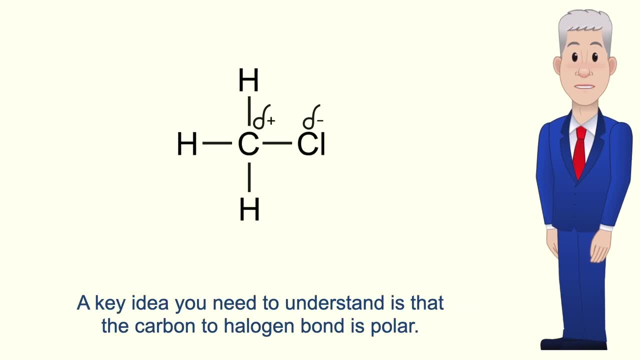 atom which is bonded to two other carbon atoms, And in tertiary haloalkanes, the halogen is bonded to a carbon atom which is bonded to three other carbon atoms. Okay now a key idea you need to understand is that the carbon to halogen bond is polar, and this polarity affects both the physical 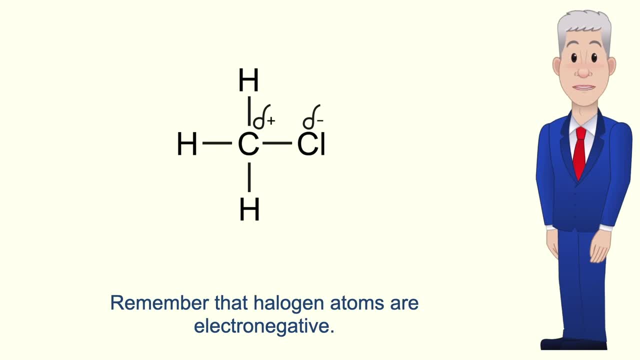 properties and reactivity of haloalkanes. Remember that halogen atoms are electronegative. This means that the pair of electrons in the covalent bond between the carbon atom and halogen atom is closer to the halogen than the carbon. Because of this, the halogen atom has a slight 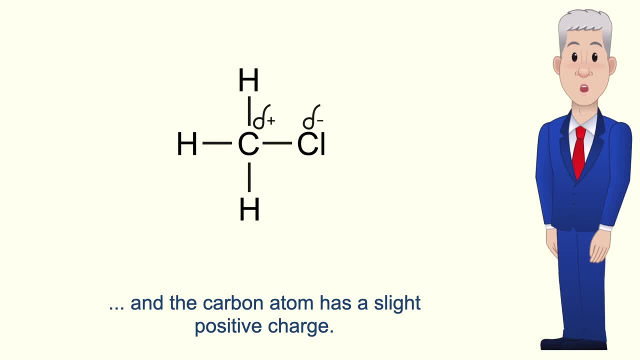 negative charge and the carbon atom has a slight positive charge. Now, in the next video, we'll start looking at how this bond polarity affects the reactivity of the haloalkanes, but we're going to finish this video by looking at their physical properties. I'm showing you here the boiling points. 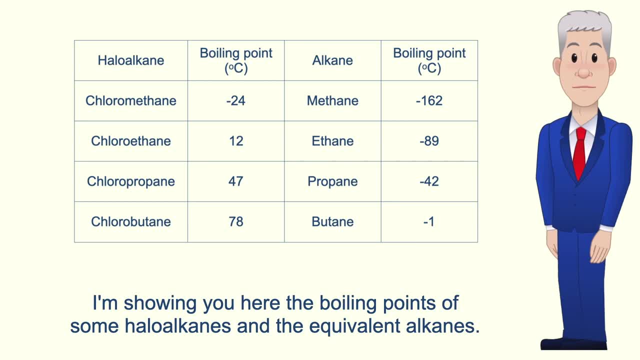 of some haloalkanes and the equivalent alkanes. The first idea you need to understand is that haloalkanes have higher boiling points than the equivalent alkanes, And this is because of the intermolecular forces. Alkanes are non-polar molecules, so the 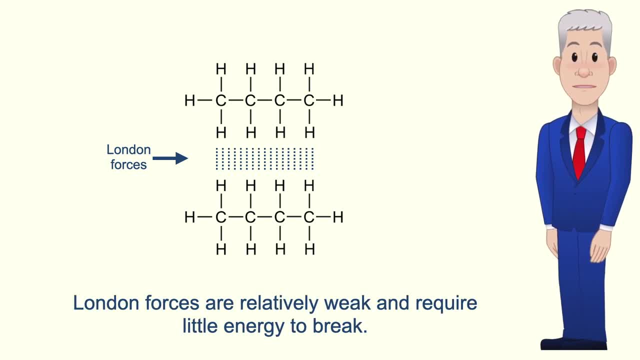 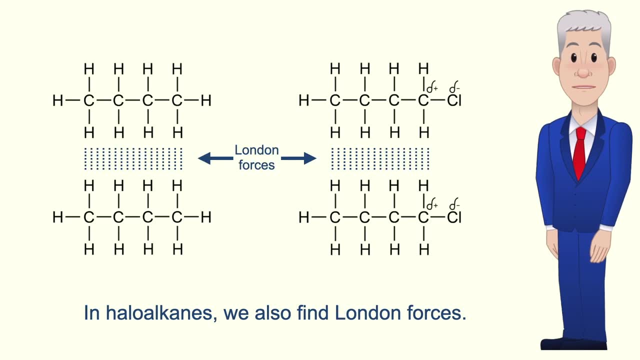 intermolecular forces are London forces. London forces are relatively weak and require little energy to break, So alkanes have relatively low boiling points. In haloalkanes we also find London forces. However, because of the polarity of the carbon to halogen bond we also find permanent 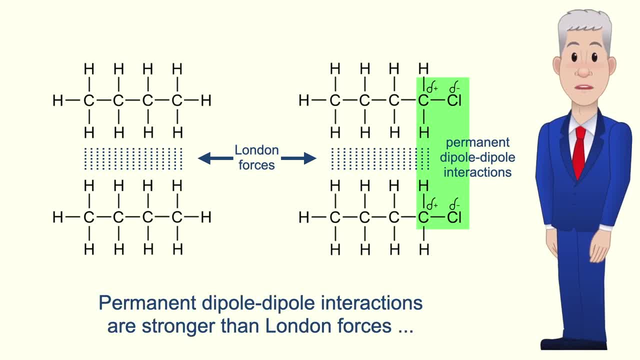 dipole-dipole interactions. Permanent dipole-dipole interactions are stronger than the polarity of the carbon to halogen bond. This is because the polarity of the carbon to halogen bond is higher than London forces and require more energy to break. So this explains. 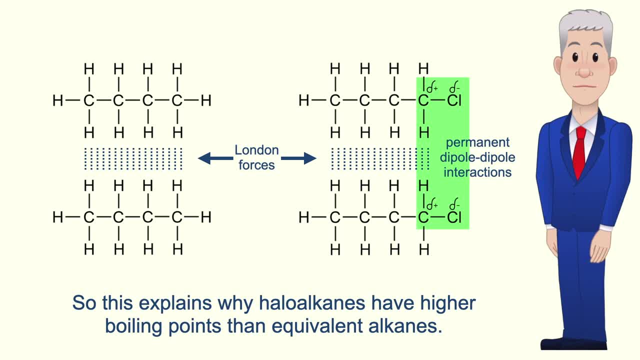 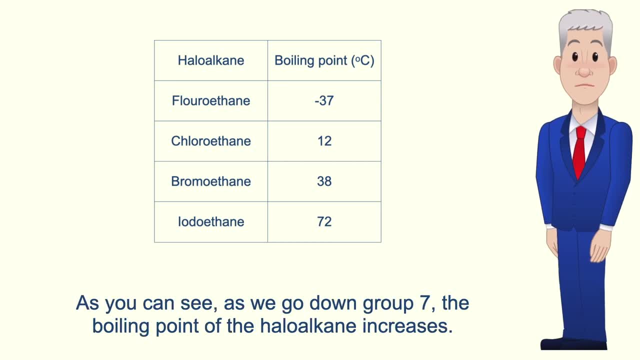 why haloalkanes have higher boiling points than equivalent alkanes. I'm showing you here the boiling points of four haloalkanes based on ethane. As you can see, as we go down group seven the boiling point of the haloalkane increases And again this is due to London forces. The number of 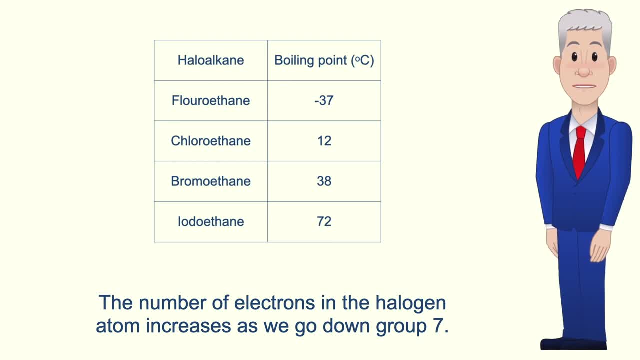 electrons in the halogen atom increases as we go down group seven And London forces are larger when there are more electrons. The number of electrons in the halogen atom increases as we go down group seven. Larger London forces require more energy to break And this explains why the